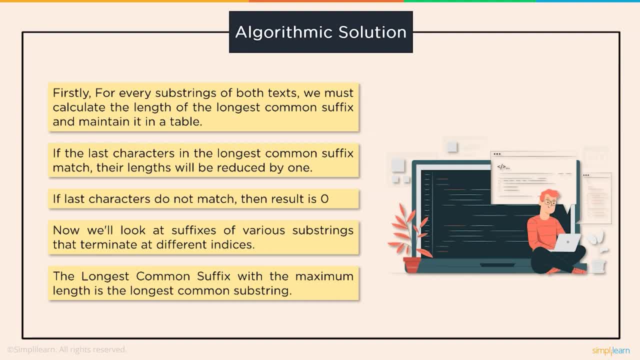 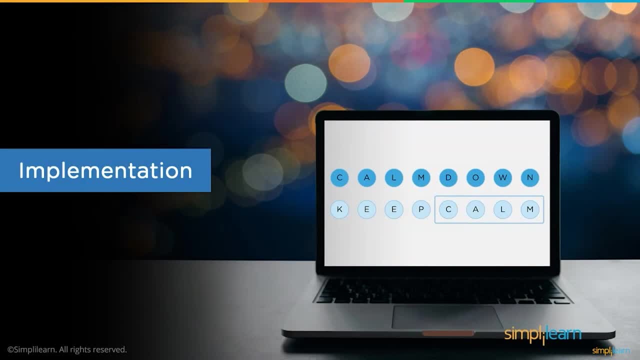 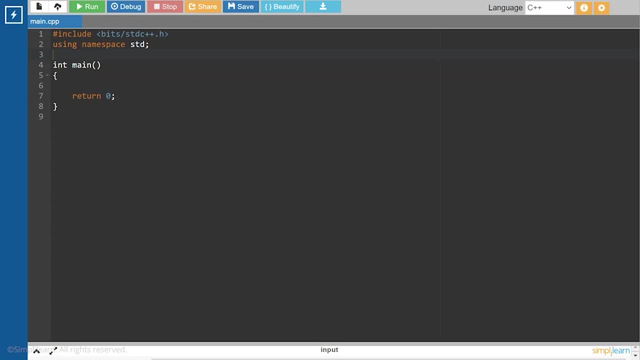 is the longest common suffix with the maximum length. We have now discussed the problem statement and the algorithmic solution to find the longest common substring. Now let's implement this solution in the code editor. We will start with a function that will return the length of. 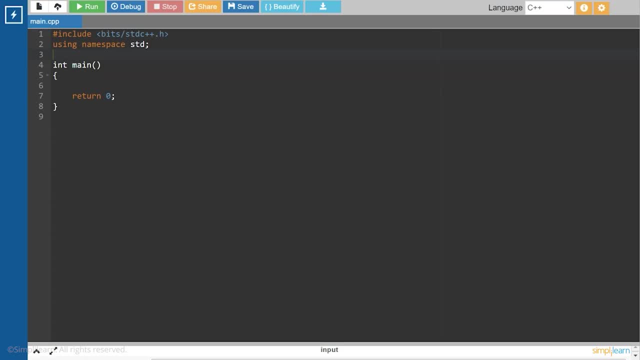 the longest common substring of a string x and y int. lcsubstr its argument as: star char x comma character pointer: y comma int. the size of the first string, x comma int. n. This will be the size of the another string, y. Now we will create a table to store the lengths of longest common suffixes of. 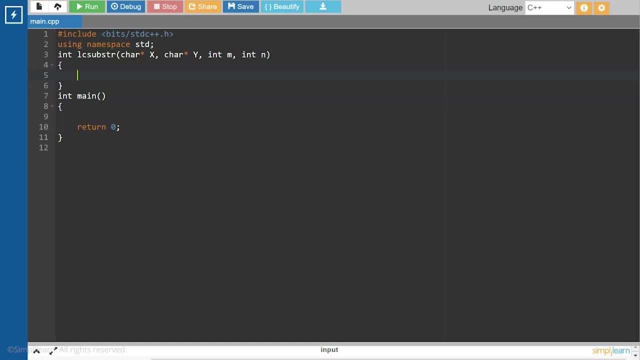 string. Now we will create a array lcsub to store the length of the longest common suffix. So int lcsub at m plus 1 and n plus 1 and another variable result equals to zero. This will be used to store the length of the longest common suffixes, So int lcsub. 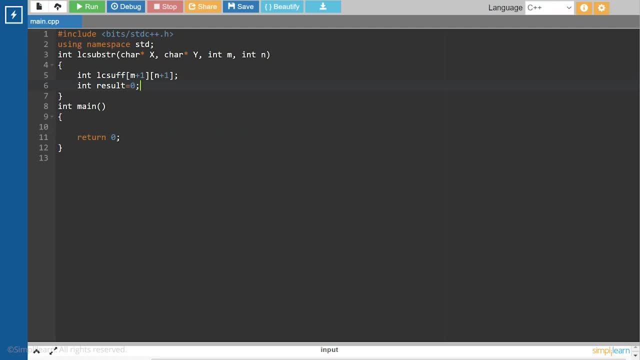 at m plus 1 and n plus 1 and another variable result equals to zero. This will be used to store the length of the longest common substring. Now we will follow the steps to build the LC suffix in the bottom-up fashion. So for int i. 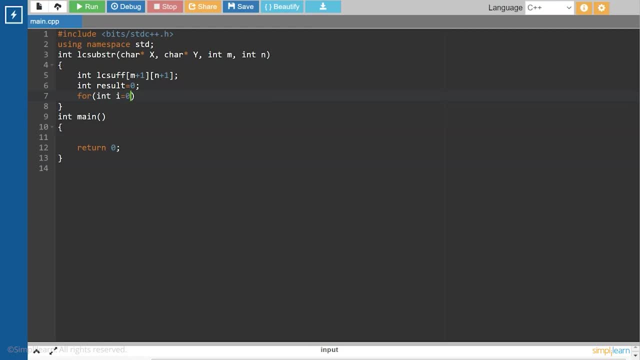 equals to zero, i less than equals to m. i plus plus Another nested loop, 4.. Int j is equals to zero, j less than equals to m, j less than equals to m, j less than equals to m and j++. now the first row and the first column entries will have no logical. 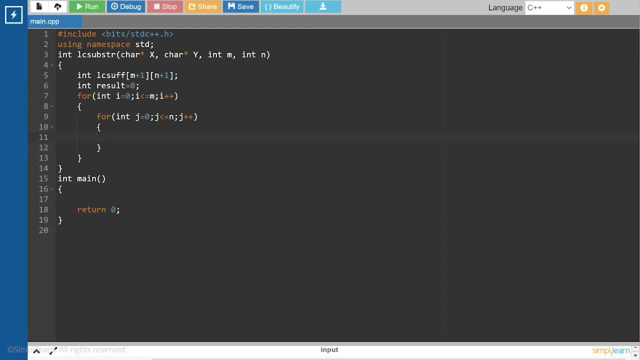 meaning they will be used only for the simplicity of the program. so if I is equals to 0 or J is equals to 0, then else is of. at I comma, J will be equals to 0. else if X at I minus 1 is equals to Y at J minus 1. 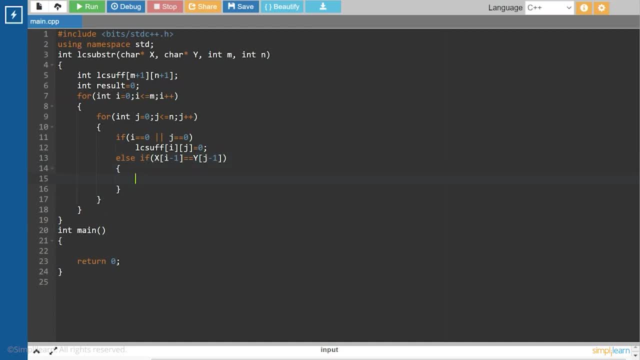 then else is of at I comma J will be equals to else is of at I minus 1. then else is of at I comma J will be equals to else is of at I minus 1 and J minus 1 plus 1, and the result will be equals to the maximum of result. 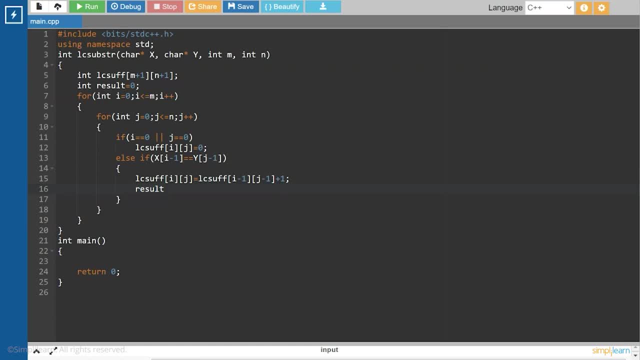 and J minus 1 plus one and the result will be equals to the maximum of result comma. else we serve at i j, else else we serve at i. j will be equals to zero and we will return result. Now let's write the main block, so we will have string: char x is equals. 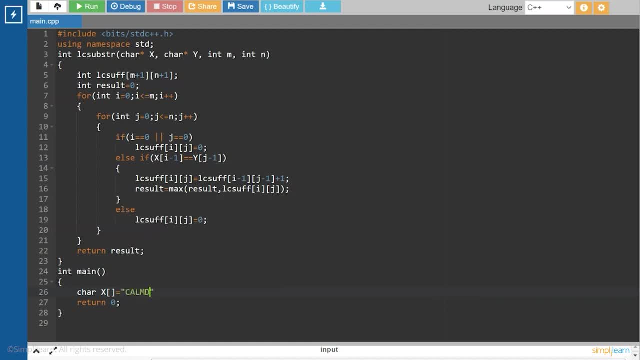 to calm down. and another string, char y is equals to keep calm. Now we will store the length n. m is equals to strln of x and int n will have strln of x of Y. Now we will print the length of longest common substring.